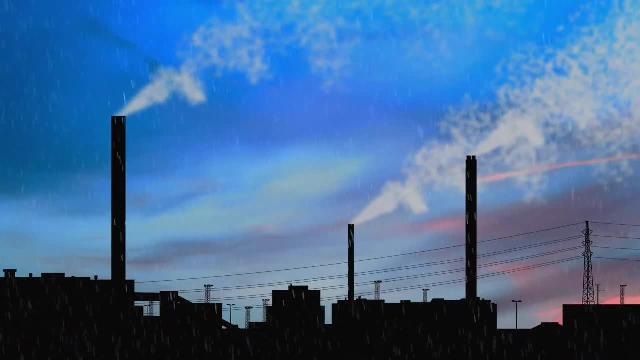 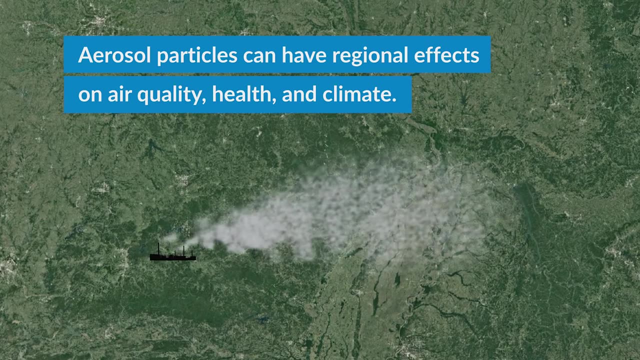 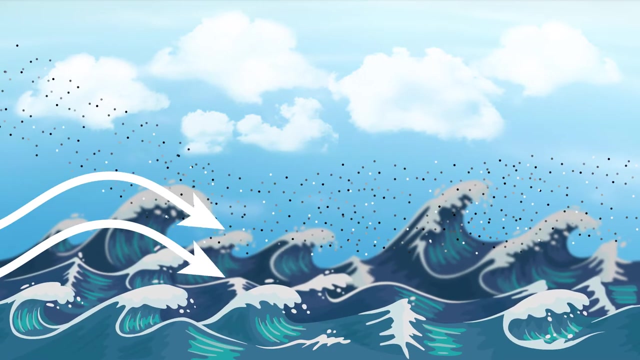 get rained out or snowed out. Their climate effect is very regional, so it's only in that region that they're going to impact either air quality or health effects or climate. Sea Spray aerosol is the largest mass of particulate matter that's ejected naturally into the atmosphere. It is responsible. 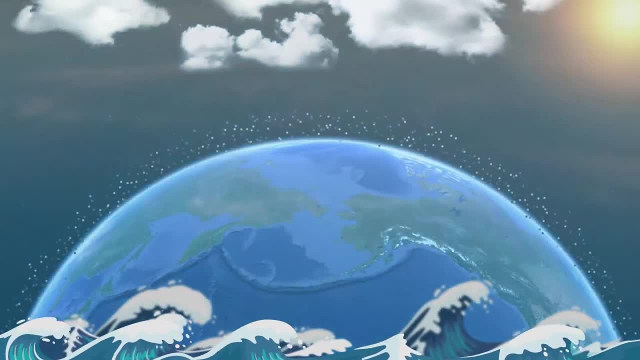 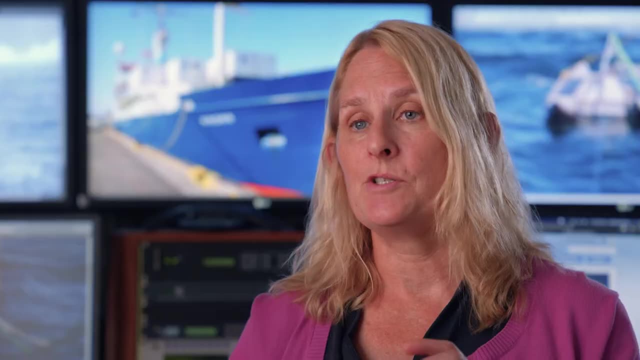 for most of the light scattering over the ocean, which is a way of reflecting radiation back to space. If you're out in the middle of the ocean, there's way fewer particles. Any change- and even if it's a small change- in those particulates has a much bigger impact. 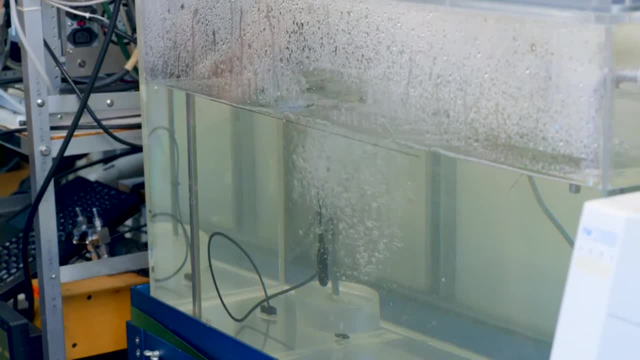 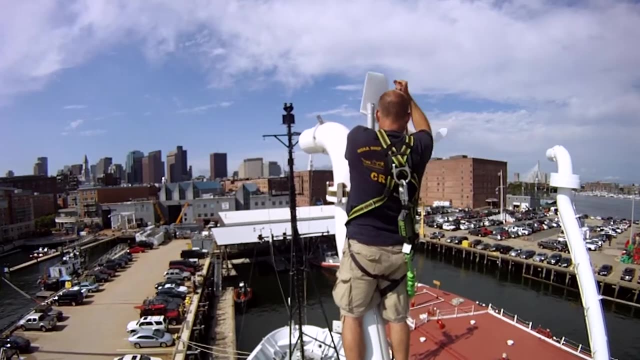 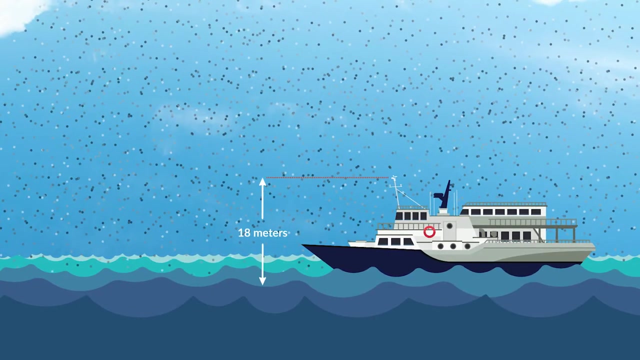 And we really want to know how these particulates are interacting, particularly with clouds. Currently, the way we sample is we have a mass that's as far forward and as high on the ship as we can get it, so that's about a height of 18 meters, But that's only looking at the very lower. 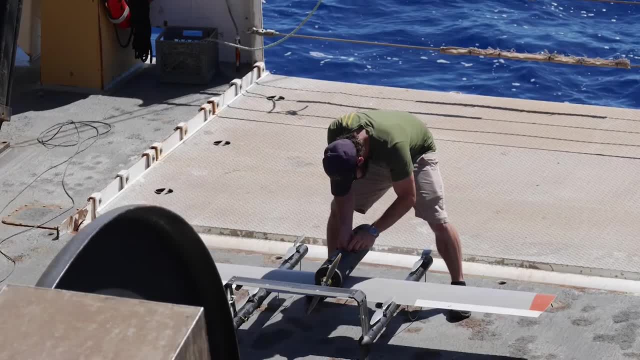 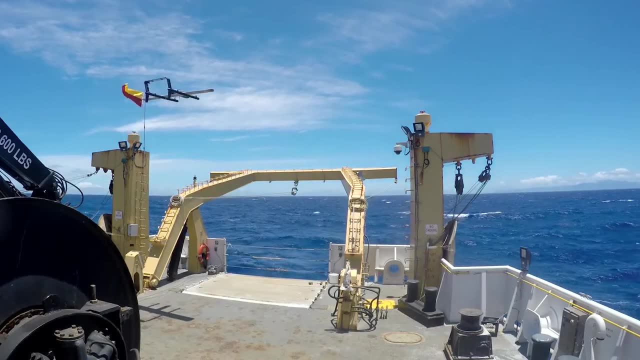 portion of the atmospheric boundary there. So we're developing an unmanned aerial vehicle in order to combine that with the measurements we get from the surface from the ship That will be used to measure the surface of the ship That will be used to measure the surface of the. 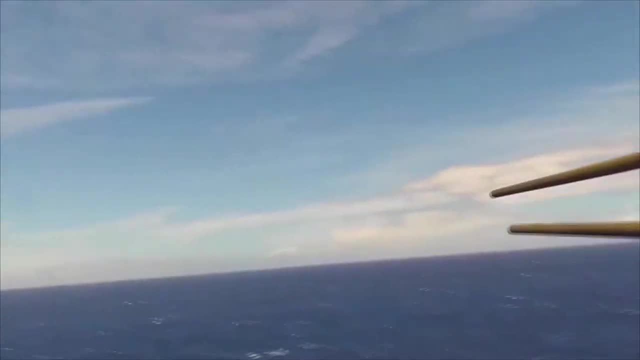 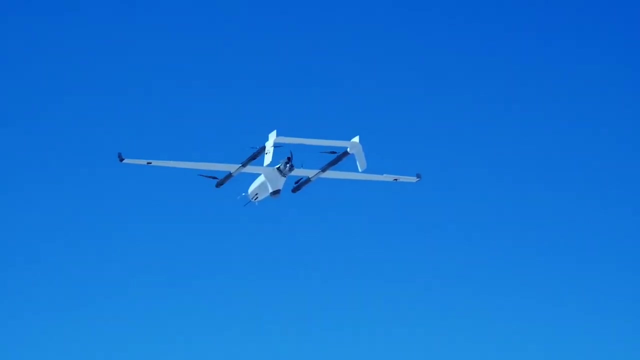 ship. We'll be able to sample the lower atmosphere sample right below cloud base. figure out what particulates are actually reaching the cloud base so that see how they impact cloud properties. We came up with a technique for measuring freshly emitted sea spray aerosol. 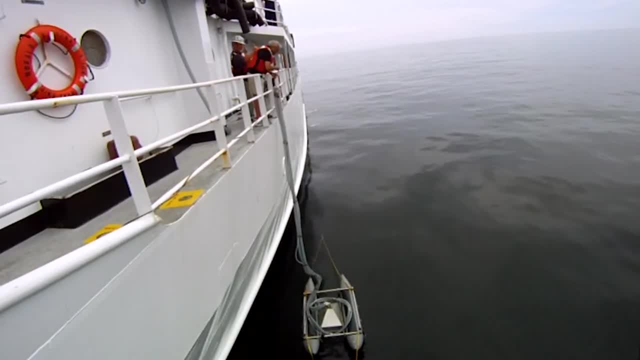 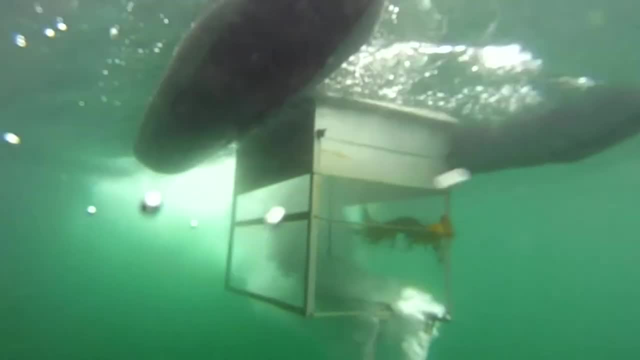 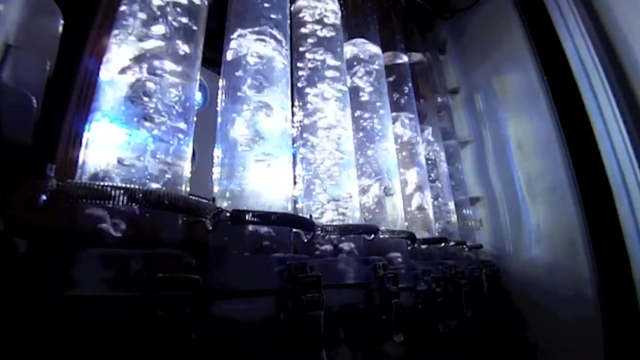 We essentially have this pontoon and this oven hood on top of it. We deploy it over the port side of the ship. We put compressed air through and they bubble at about three quarters of a meter below the surface To imitate the wind-driven production of sea spray. These bubbles take up organics and 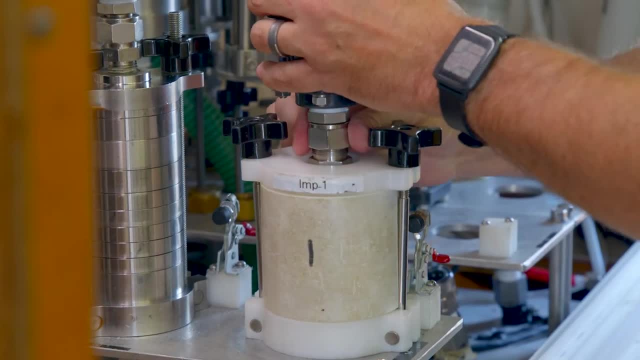 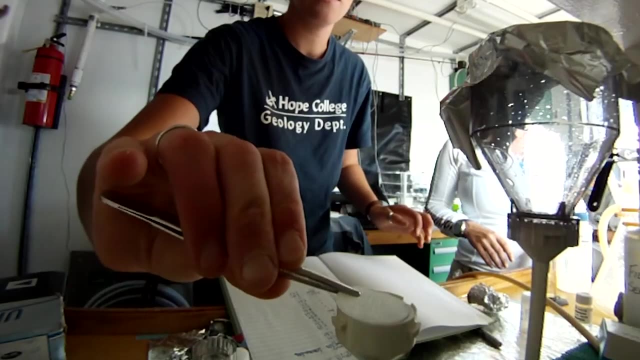 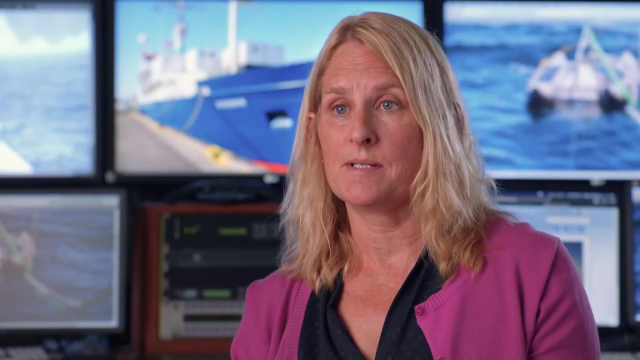 inorganics as they are rising into the atmosphere. It's important to know how the sea spray aerosol are impacting cloud properties, because it could be a way to help cool the planet. The emphasis for NOAA is on long-term observations. We're not just sitting at. 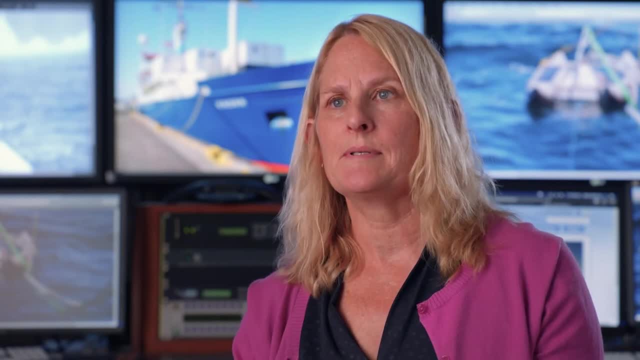 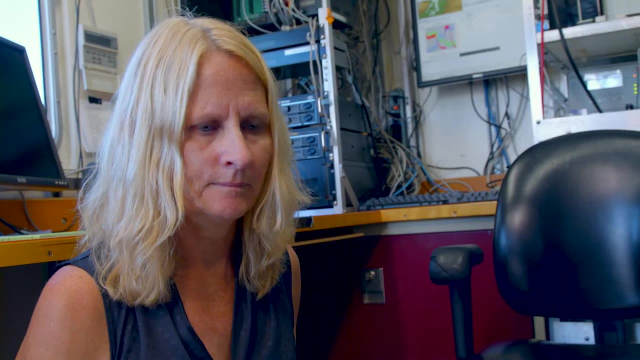 one spot for 20 years, but we're doing the same type of work in many different regions, trying to understand how it varies regionally and how that impacts the global picture.